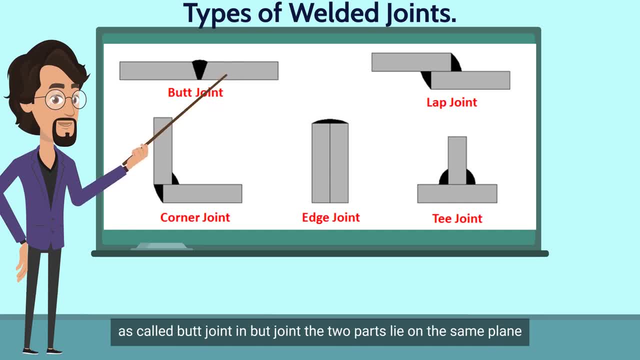 The joint which is formed by placing the electrode, The joint which is formed by juntoing the terrific circuit, The joint which is formed by placing the electrode And the joint whichario can be準備d with the end of the зал joint. 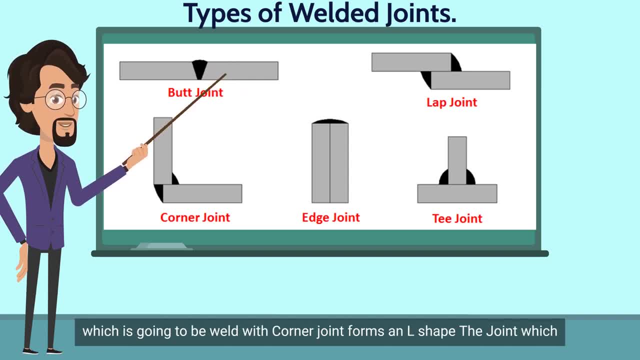 The joint which is formed by placing the soldered electrode on the slide. The joint which is formed by placing the unter goalylie Natory section of metal. The joint of the grip together at right a l shouldlos angle. The joint which is formed by placing the corner of the two parts. 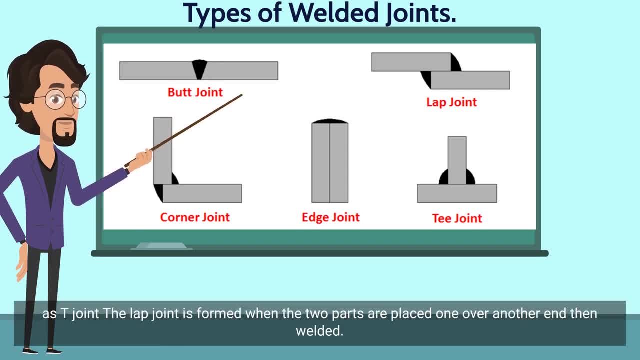 The side joint can be wirt thi Gel placed at a物 angle. This joint, which is going to lead lett with one end connected to it at the right angle, t-joint. the lap joint is formed when the two parts are placed one over another end, then welded it may. 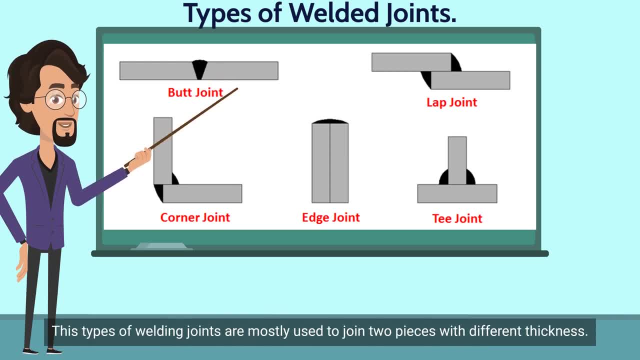 one-sided or double-sided. this types of welding joints are mostly used to join two pieces with different thickness. the joint formed by welding the edges of two parts together are called edge joint. this joint is used where the edges of two sheets are adjacent and are approximately parallel planes at the point of welding. it cannot be used in stress and pressure application because 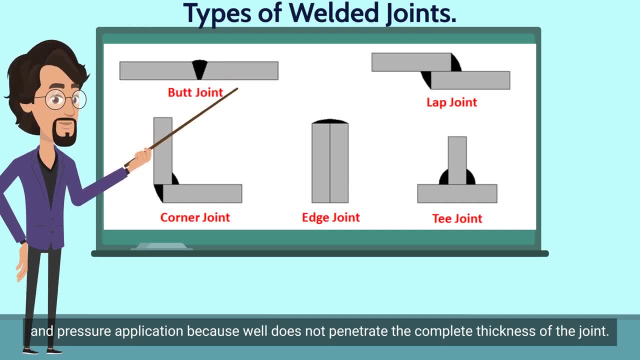 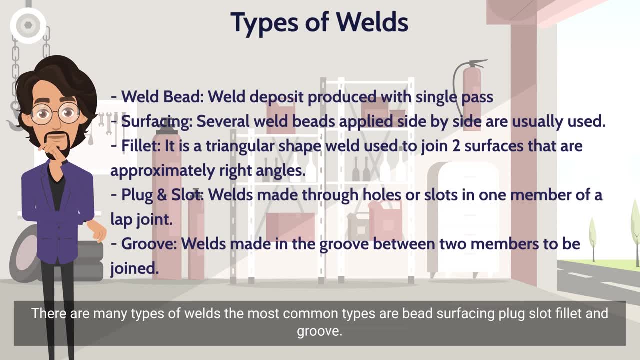 weld does not penetrate the complete thickness of the joint. there are many types of welds. the most common types are bead, surfacing, plug, slot, fillet and groove. a weld is a well deposit produced by a single pass. with welding it may narrow or wide depending on the side to side movement by the 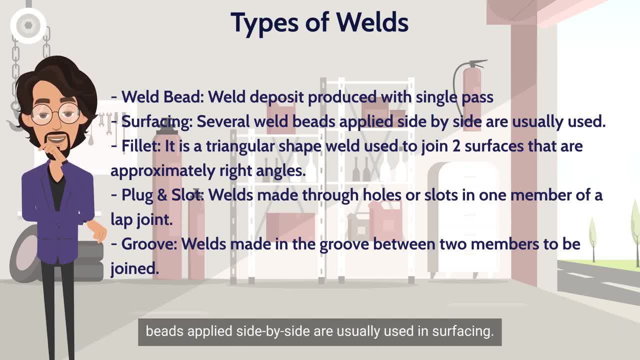 welder. several weld beads applied side by side are usually used in surfacing. a fillet weld is triangular in shape and this weld is used to join two surfaces that are approximately at right angles. plug-in slot welds are made through holes or slots in one member of a lap. joint groove welds are simple 12s made between two members to be joined. 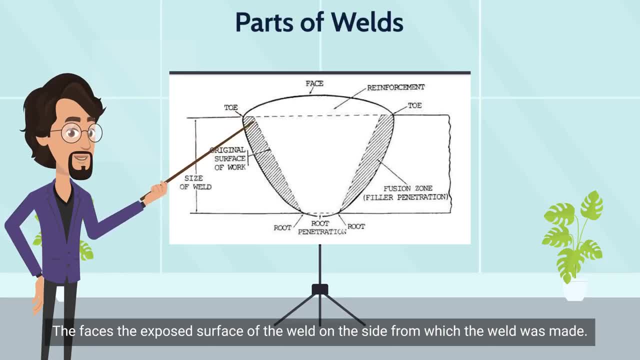 the face is the exposed surface of the weld. on the side from which the weld was made, the toe is the junction between the face of the weld and base metal. the root of a weld includes the points at which the back of the weld intersects the base metal. 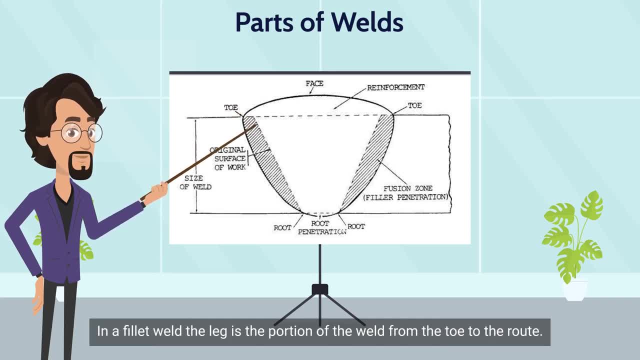 surface. in a fillet weld, the leg is the portion of the weld from the toe to the root. in a fillet weld, the throat is the distance from the root to a point on the face of the weld along the line perpendicular to the face of the weld. 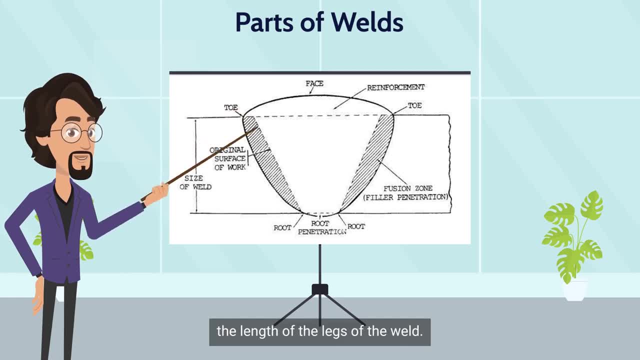 The size of the fillet weld refers to the length of the legs of the weld. Reinforcement is the weld metal in excess of the metal necessary to fill a joint. The fusion zone is the region of the base metal that is actually melted. The heat affected zone refers to that portion of the base metal that has not been melted. 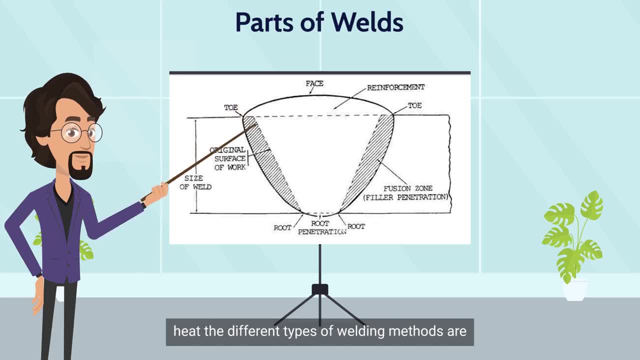 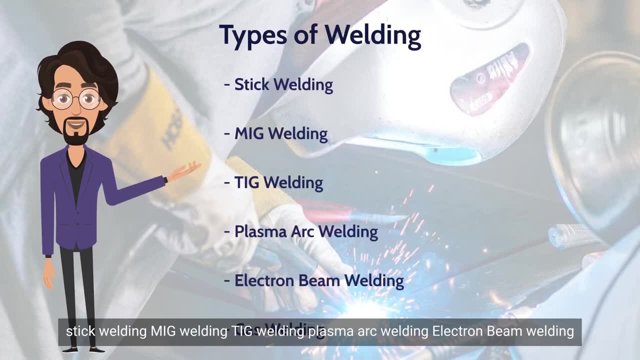 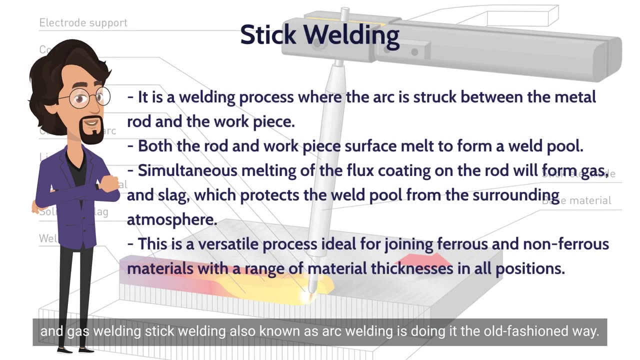 However, properties of the metal are altered by the welding heat. The different types of welding methods are Stick welding, MIG welding, TIG welding, plasma arc welding, electron beam welding and gas welding. Stick welding, also known as arc welding, is doing it the old fashioned way. 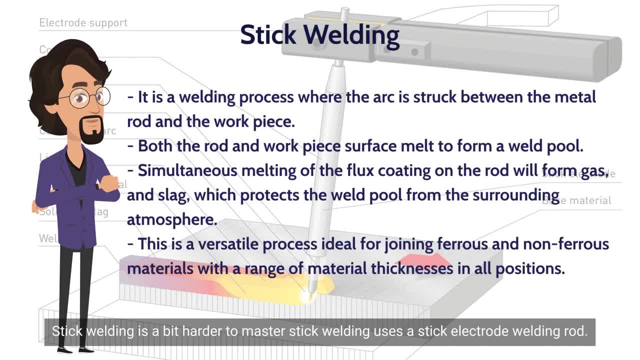 Stick welding is a bit harder to master. Stick welding uses a stick electrode welding rod. It is a process in which the arc is struck between the metal rod and the workpiece. Both the rod and workpiece surface melt to form a weld pool. 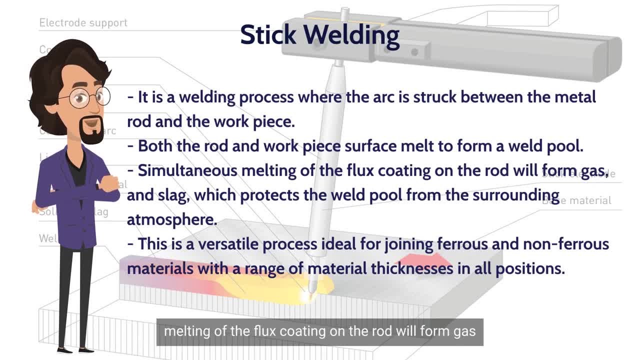 Simultaneous melting of the flux, coating on the rod will form gas and slag, which protects the weld pool from the surrounding atmosphere. This is a versatile process Ideal for joining ferrous and non-ferrous materials with a range of material thicknesses in all positions. 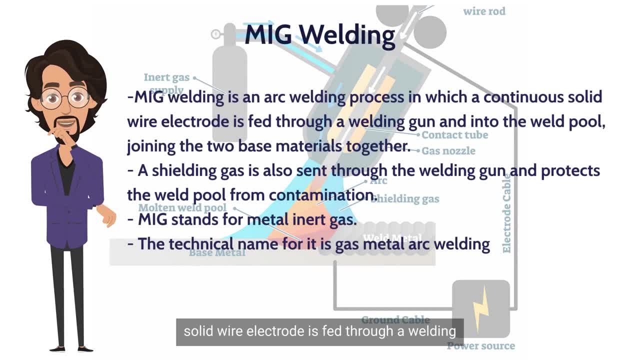 MIG welding is an arc welding process in which a continuous solid wire electrode is fed through a welding gun and into the weld pool, Joining the two base materials together. A shielding gas is also sent through the welding gun and protects the weld pool from contamination. 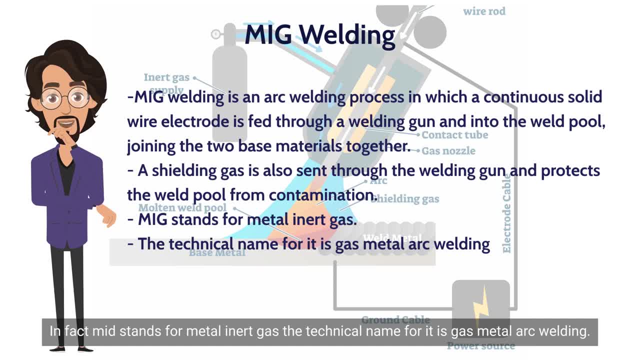 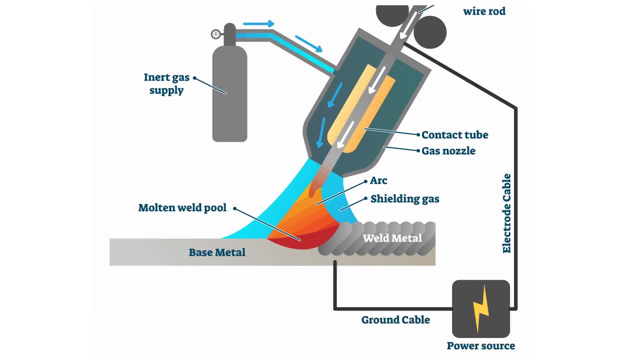 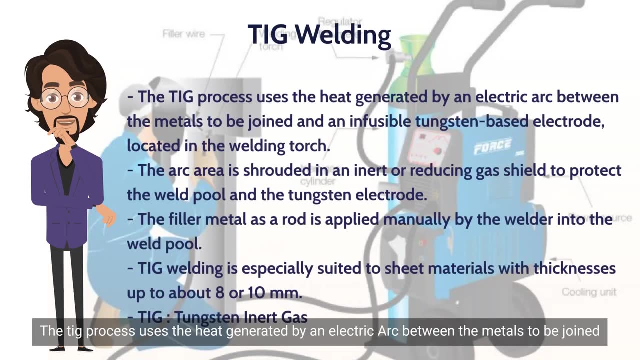 In fact, MIG stands for metal inert gas. The technical name for it is gas metal arc welding. The TIG process uses the heat generated by an electric arc between the metals to be joined and an infusible, tungsten-based electrode located in the welding torch. 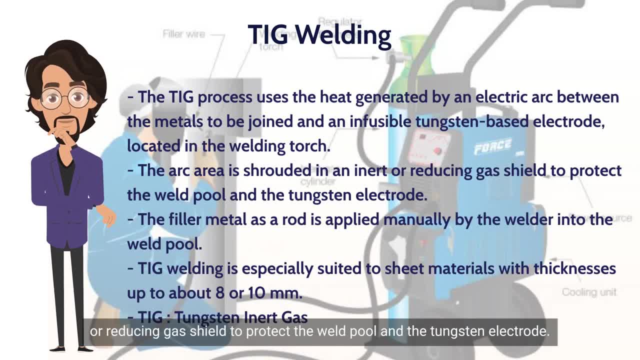 The arc area is shrouded in an inert ore reducing gas shield to protect the weld pool and the tungsten electrode. The filler metal as a rod is applied manually by the welder into the weld pool. TIG welding is especially suited to sheet materials with thicknesses up to about 8 or 10 mm. 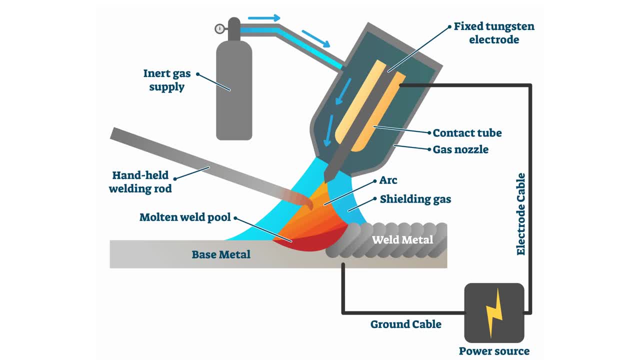 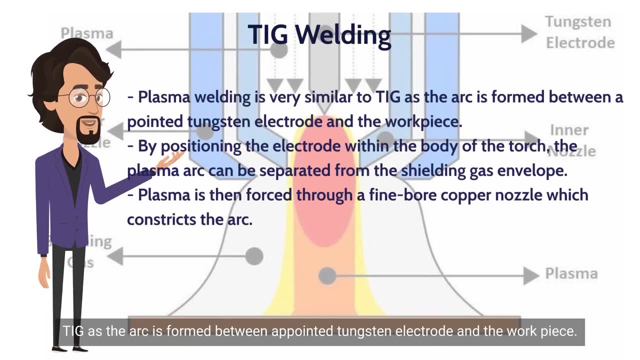 Plasma welding is very similar to TIG, as the arc is formed between a pointed tungsten electrode and the workpiece. However, by positioning the electrode within the body of the torch, the plasma arc can be separated from the shielding gas envelope. Plasma is then forced through a fine-bore copper nozzle, which constricts the arc. 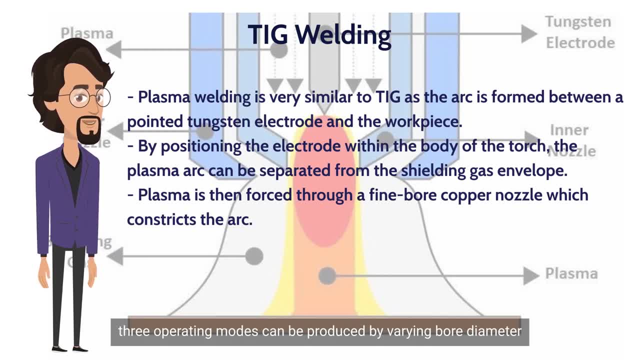 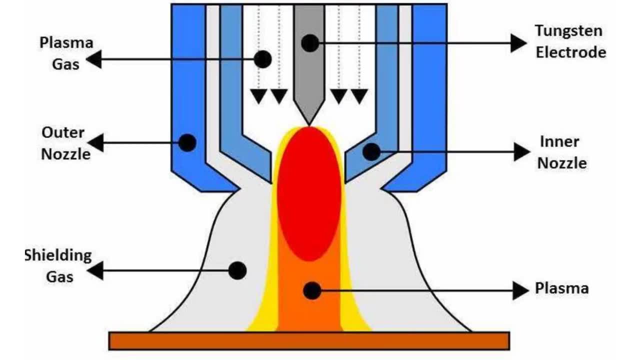 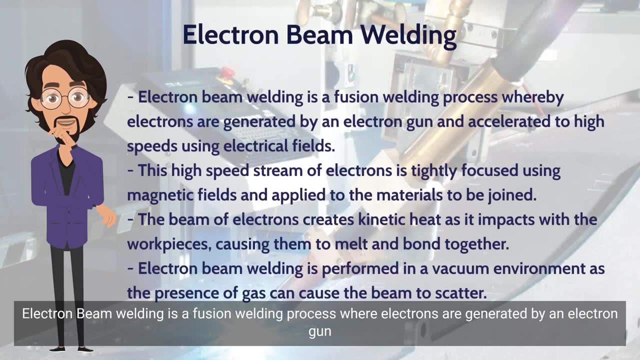 Three operating modes can be produced by varying bore diameter and plasma gas flow rate. Electron beam welding is a fusion welding process where electrons are generated by an electron gun and accelerated to high speeds using electrical fields. This high-speed stream of electrons is tightly focused, using magnetic fields and 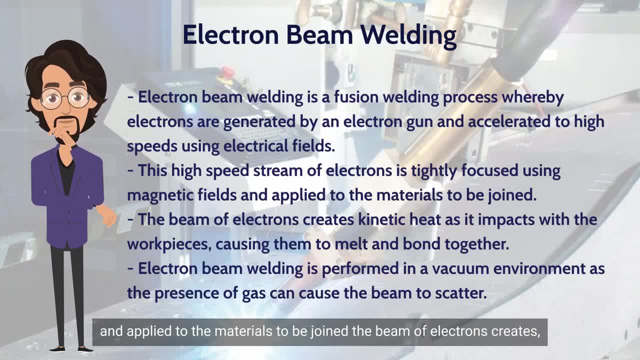 applied to the materials to be joined. The beam of electrons creates kinetic heat as it impacts with the workpieces, causing them to melt and bond together. Electron beam welding is performed in a vacuum environment, as the presence of gas can cause the beam to scatter. 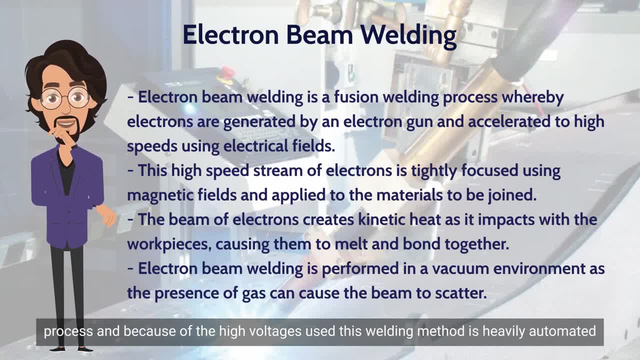 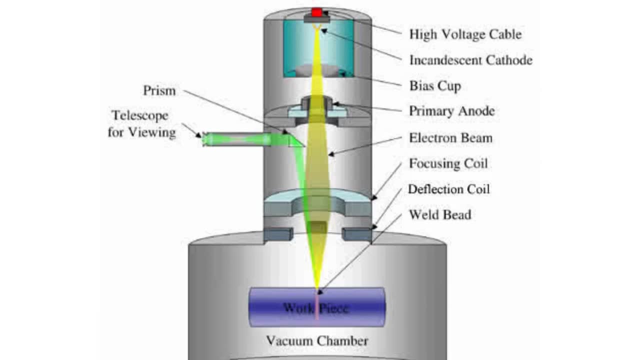 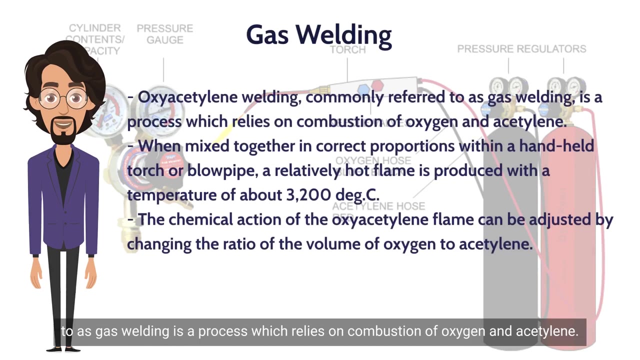 due it being a vacuum process and because of the high voltages used, This welding method is heavily automated and computer controlled. As a result, specialized fixtures and CNC tables are used to move the workpieces inside the welding vacuum chamber. Oxi-acetylene welding, commonly referred to as gas welding. 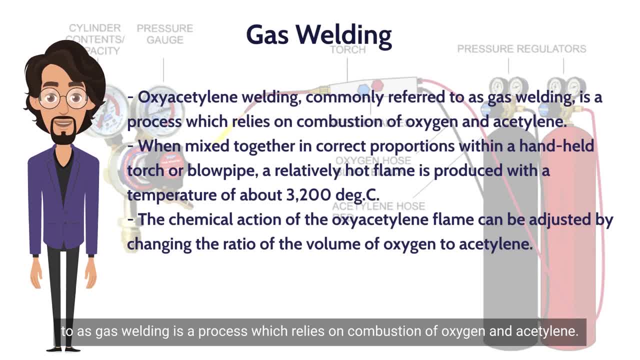 is a process which relies on combustion of oxygen and acetylene. When mixed together in correct proportions within a hand-held torch or blowpipe, a relatively hot flame is produced, with a temperature of about 3200 degrees Celsius. The chemical action of the oxy-acetylene flame can be adjusted by changing the ratio of the volume of oxygen to acetylene. 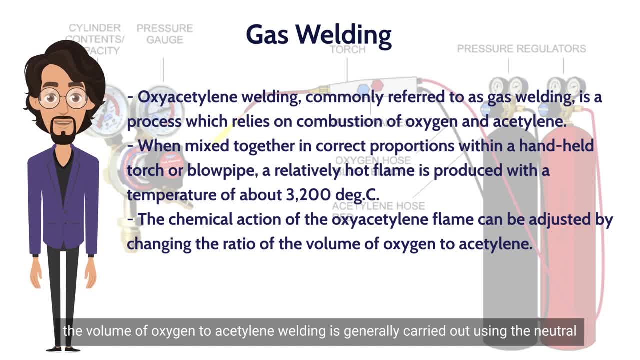 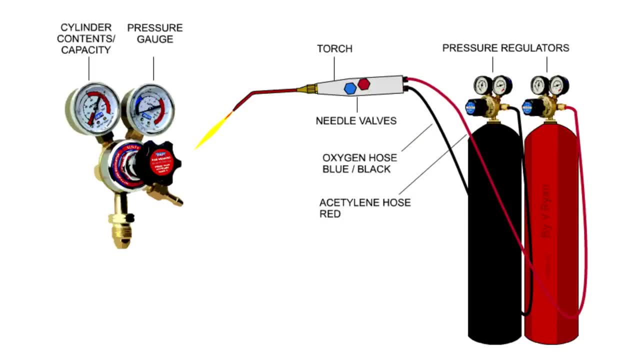 Welding is a process of combustion of oxygen and acetylene. The chemical action of the oxy-acetylene flame can be adjusted by changing the ratio of the volume of oxygen to acetylene. Welding is generally carried out using the neutral flame setting, which has equal quantities of oxygen and acetylene.